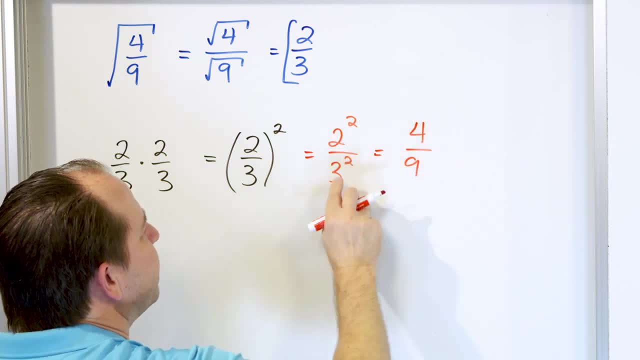 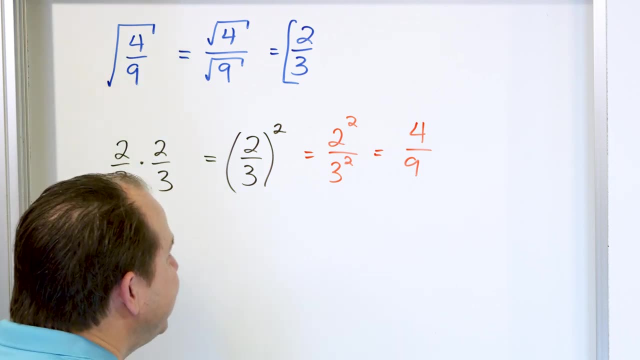 the same thing, And what you get when you multiply it out is four, ninths, because this is four and this is nine, And so when you square the answer, you get back what you started with. Now I'm going to tell you that the most important thing to this lesson is to know that when you have a radical 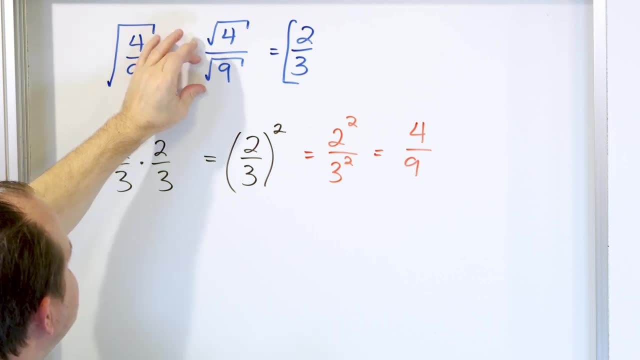 you break it up into a radical of the numerator and a radical of the denominator. You break it apart. But I also want to call your attention to what you're really doing here is you're like taking the square root and you're applying it to the top and you're applying it to the bottom, But 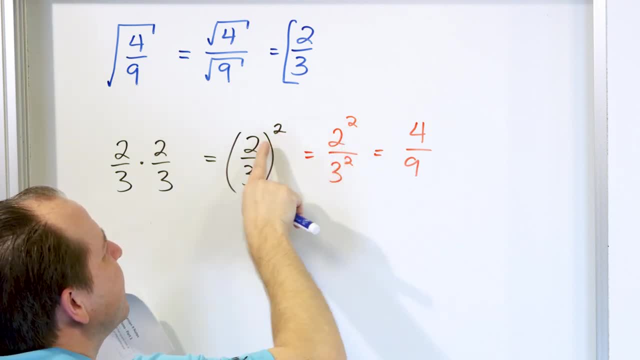 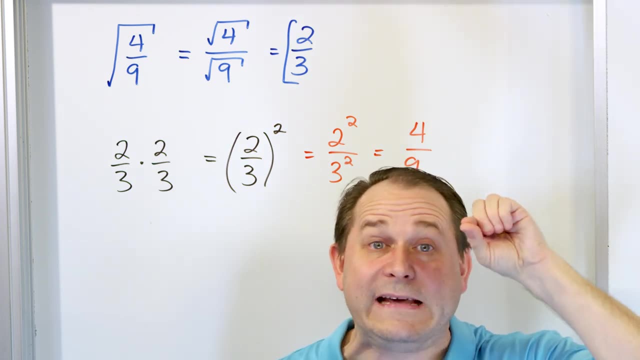 when we checked our answer notice, when we had this exponent, we applied it to the top and then we applied it to the bottom. Doesn't that look similar? That when you have an exponent applied to a fraction, you take the exponent and you apply it to the top and the bottom, And then I just told. 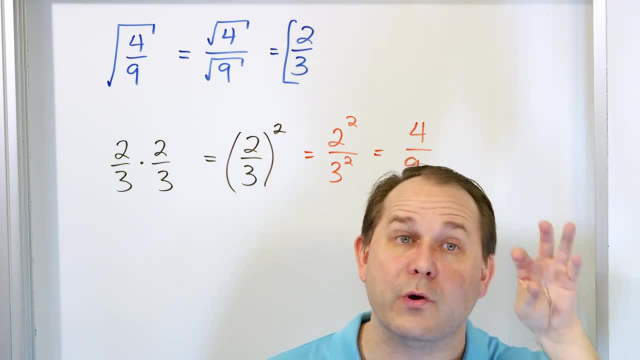 you that if you have a radical applying to a fraction, you apply it to the top and apply it to the bottom. So I'm not going to get into the full glory of the details here, but let me just tell you that the reason that you apply radical to the numerator and the denominator separately is: 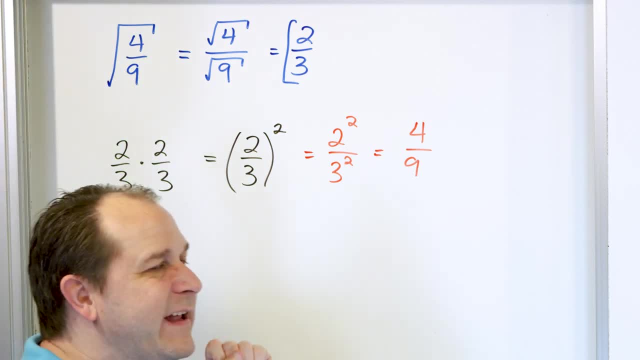 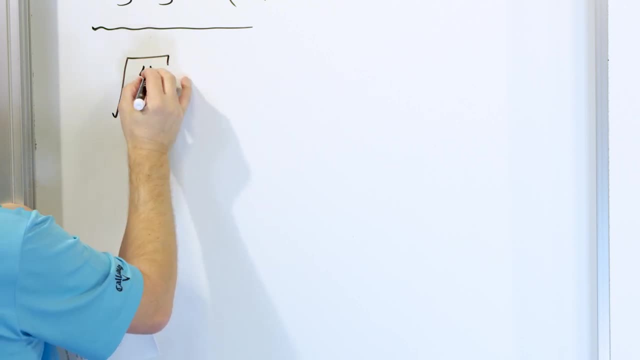 because all of these radicals can be written as exponents. I'm going to say that again because it's something that you don't know And it's something this is not the point of this lesson, but I want to show you that the square root of four ninths you're going to learn later in math. 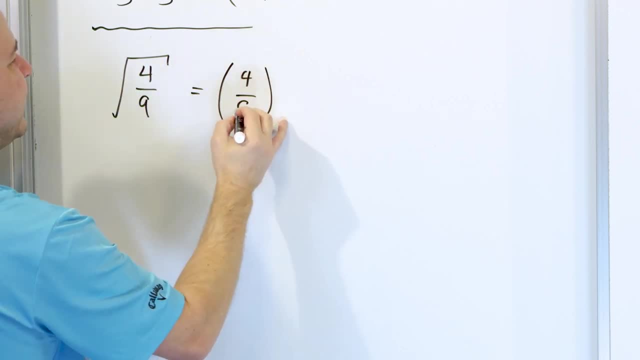 that all of these square root symbols that you've been writing down. they're exponents, but they're not exponents with whole numbers, They're exponents of fractions. In this case, the square root operation is actually an exponent of one half, The cube root operation. 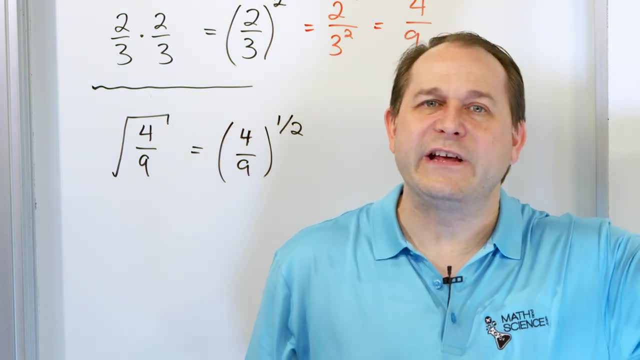 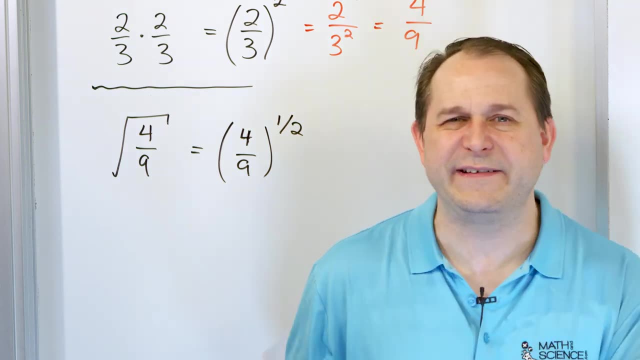 it's actually one third. If you have a fourth root, it's actually an exponent of one fourth, and so on and so on. So every square root, think about it, every square root that you've ever seen, any of them that I've written down. you could replace it by just wrapping the thing to an. 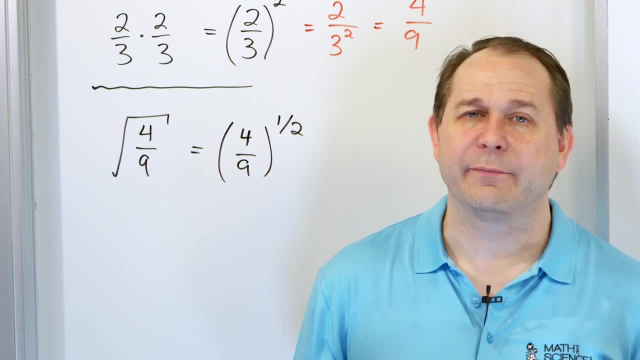 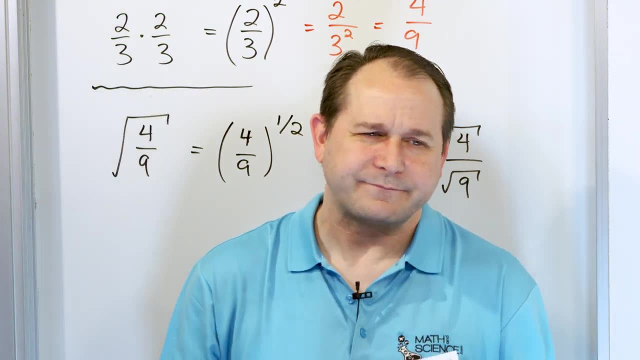 exponent of one half. As to why it's an exponent of one half, that is a lesson for another day. The point is not to teach you that, but to the bottom. So you see students, including me. when I first learned this stuff, I thought that math was. 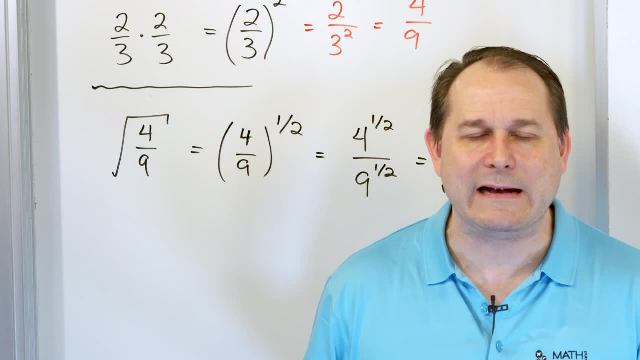 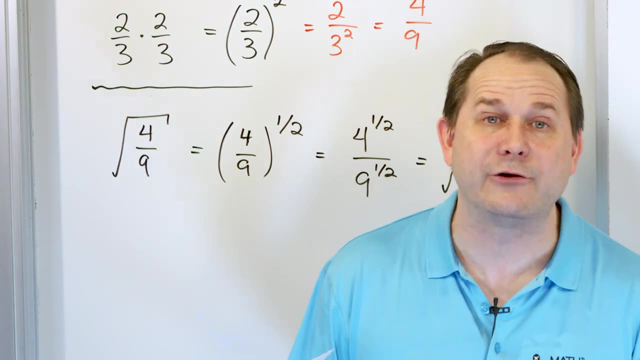 it's a collection of a million different rules and it was so hard to keep them all in my head. But you can eliminate all of that worry about all the rules if you recognize the larger pattern of what you're looking at, These things called exponents. they're everywhere. We have positive 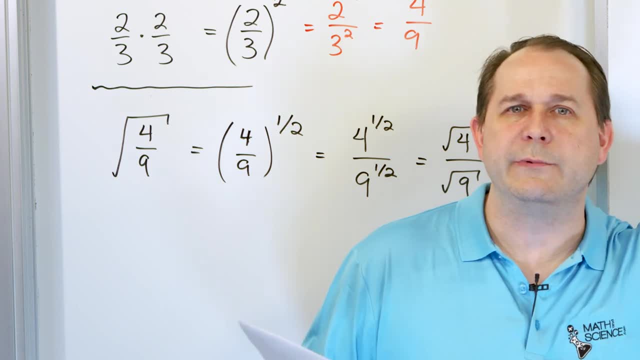 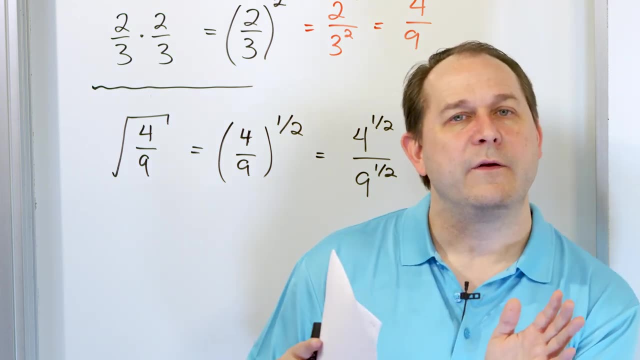 exponents that we've already learned about, like three squared and three cubed and three to the fifth and three to the eighth. We've also learned about exponents with a power of zero. We've also learned about exponents with negative exponents: three to the negative one, three to the 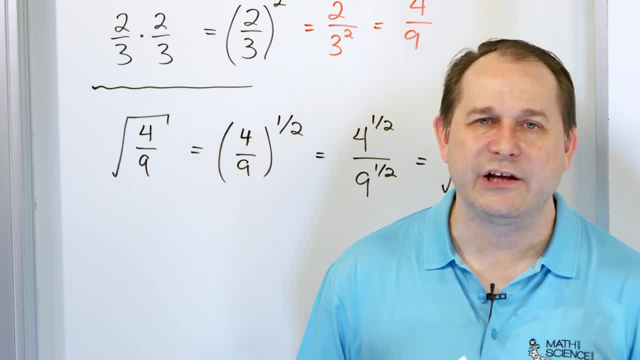 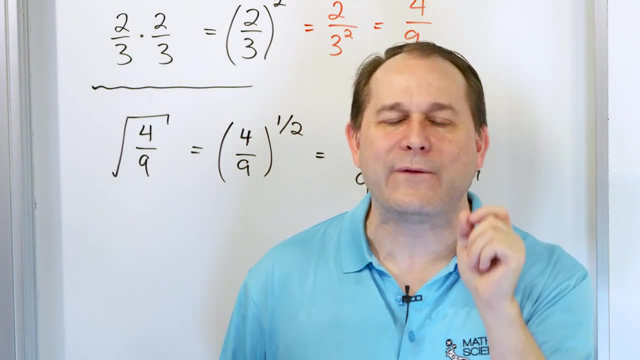 negative two. three to the negative three. We've learned about those And now I'm just telling you that exponents can also be fractions. In this case, I wrote it down as an exponent of one half, And any fractional exponent is just a radical. If it's a one half exponent, it's called a square. 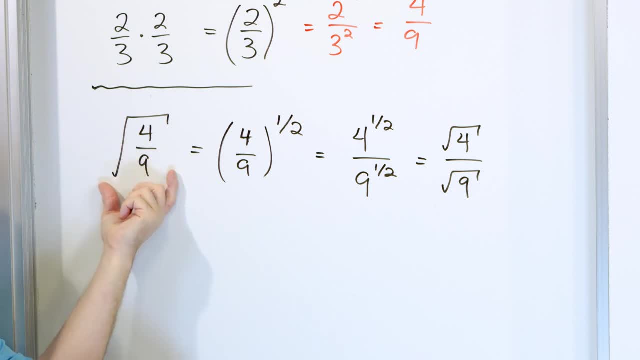 root. We have a new symbol for that that we now know. This is this checkmark thing. but it's the same thing as a fractional one half exponent. If we have a cube root, we write it down as a one third power exponent. If it's a fourth root, it's a one fourth power exponent, If it's a one third. 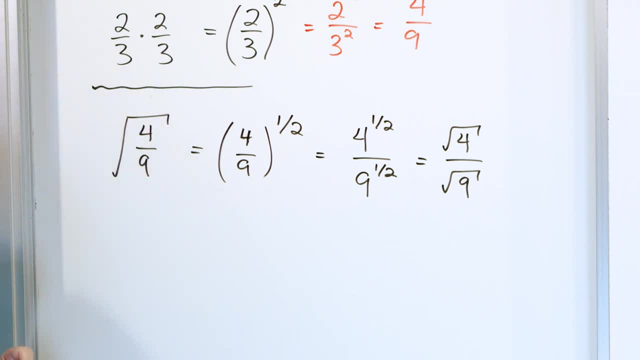 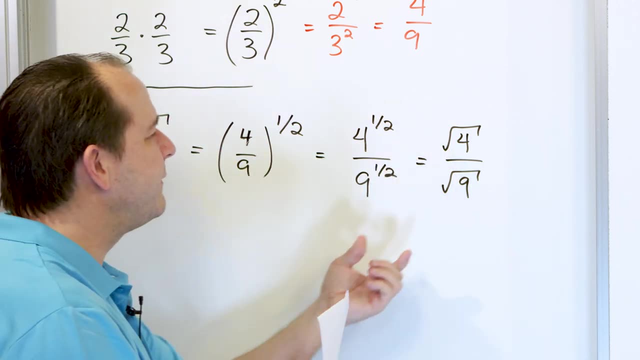 exponent. If it's a fifth root, it's a one-fifth power exponent, Radical form, because these two things are equivalent. that means that these radicals can be applied to the numerator and denominator and broken up. So I guess what I'm trying to say is: I was frustrated as a student. 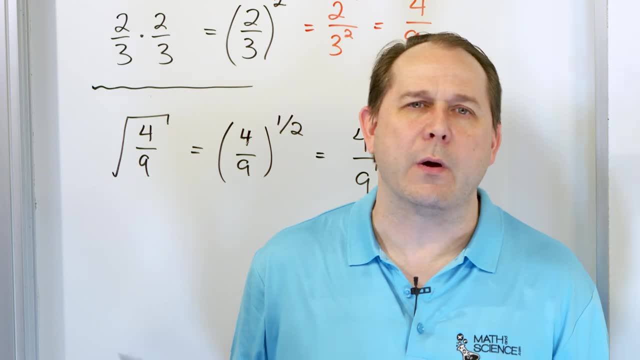 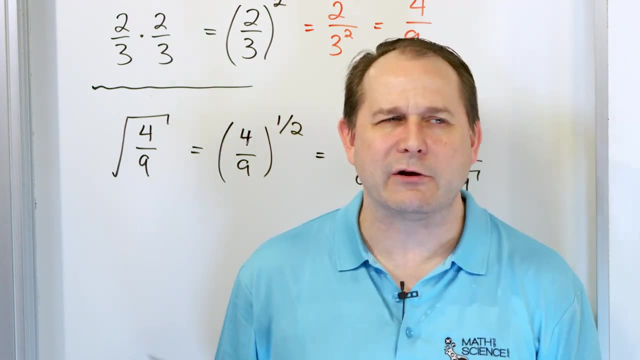 because I thought: where do all of these rules of radicals come from? Why can I, or how can I apply it, this giant radical over a fraction to the numerator and the denominator, Like: how is that legal? How do you know it's legal And nobody ever taught me until I don't know. 9th, 10th, 11th, 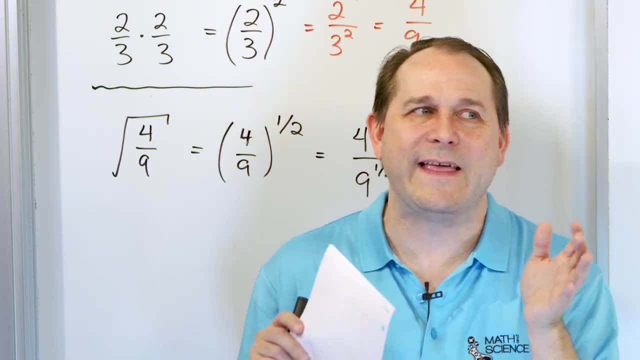 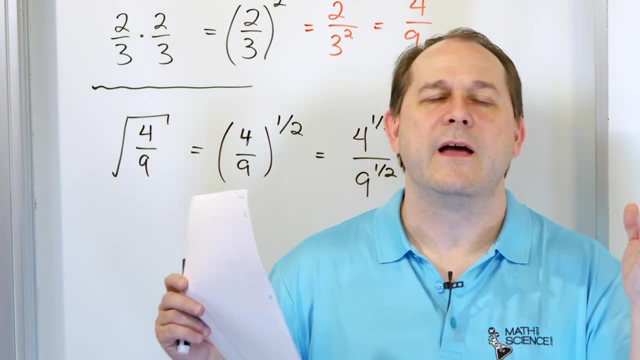 grade- maybe college- that they were fractional exponents and they just obeyed the rules of exponents. You don't put that together until later. I don't want you to see math as a collection of a million different rules. There are exponents, We have positive exponents, We have negative. 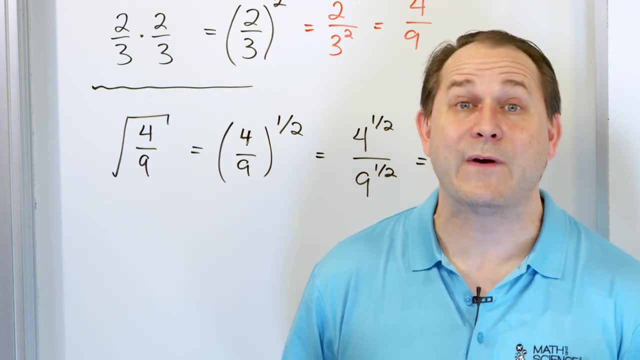 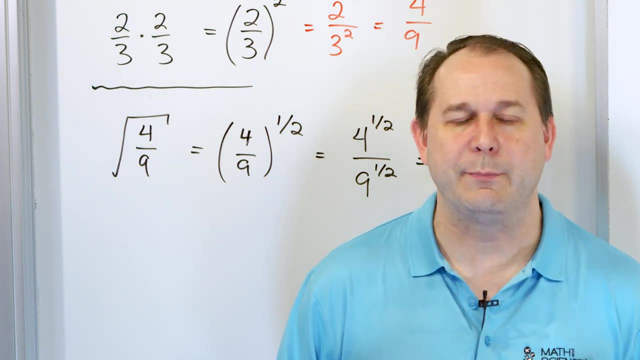 exponents. We have exponents that are zero. And now I'm telling you, we have fractional exponents, but we call them square roots if they're a one-half exponent. We call them cube roots if they're a one-third exponent. So that's why we break these radicals up and apply them to the numerator and the denominator. 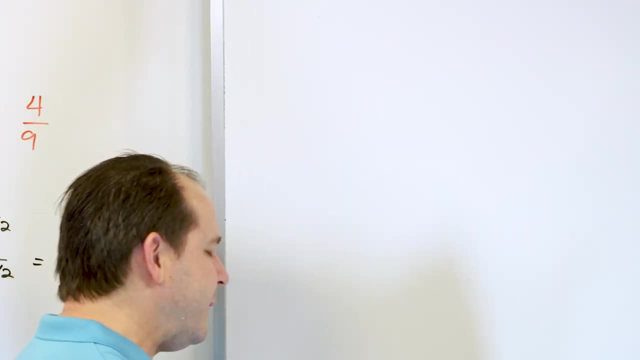 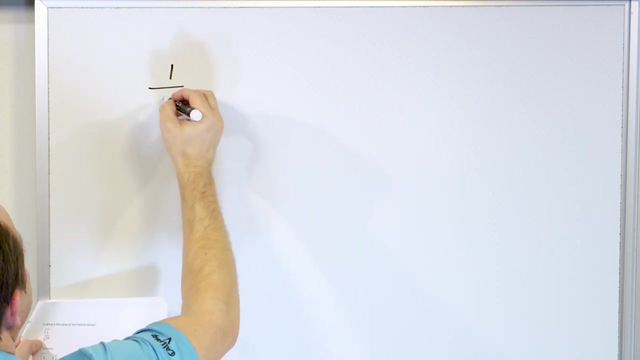 All right, with all of that out of the way, we can finally work. problem number two: I know I do a lot of talking about some of this stuff, but it's because I get so frustrated, remembering how I was confused, and I don't want you to be confused. So, diffractions, And so what do you have here? 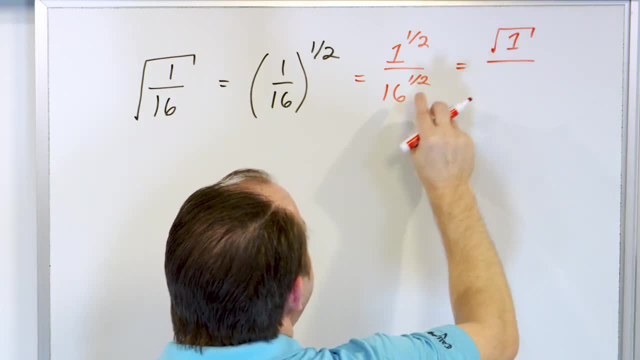 This is the square root of 1, because that's what a one-half power is. And this is the square root of 16, because that's what a one-half power is. And what is the square root of 16?? What is the square root of 1?? 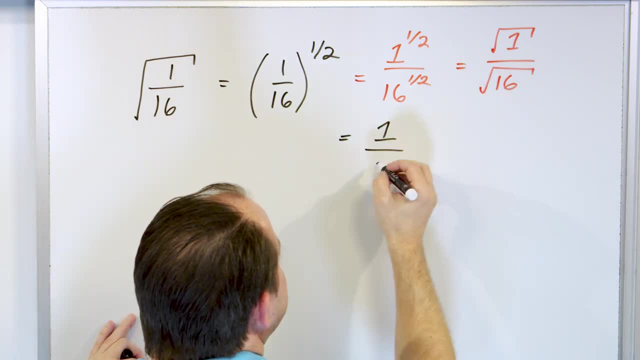 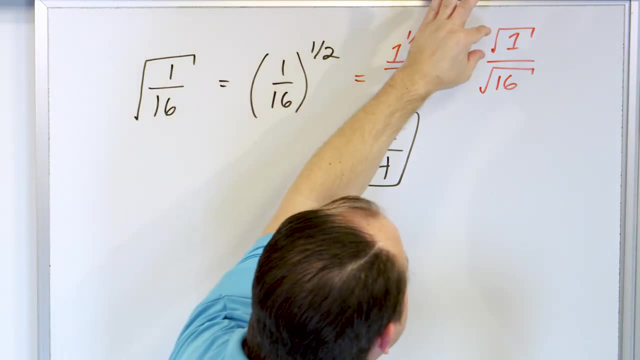 Well, it's just 1, because 1 times 1 is 1.. What is the square root of 16?? It's 4, because 4 times 4 is 16.. So the answer is 1-fourth. You take this radical and you apply it to the numerator and the denominator. 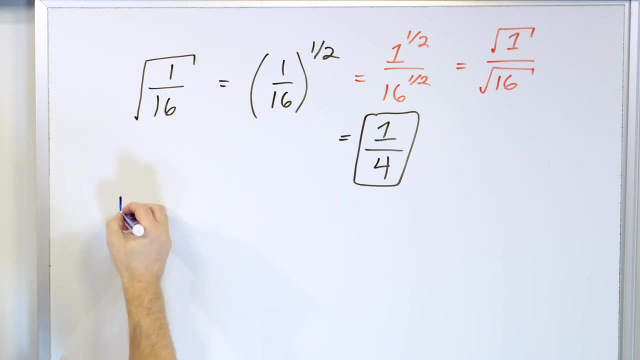 You get 1-fourth. We're not going to check every problem, but let's check it 1-fourth times itself: 1 times 1 is 1.. 4 times 4 is 16.. So, yes, this is the correct answer, because we get back what we started with. 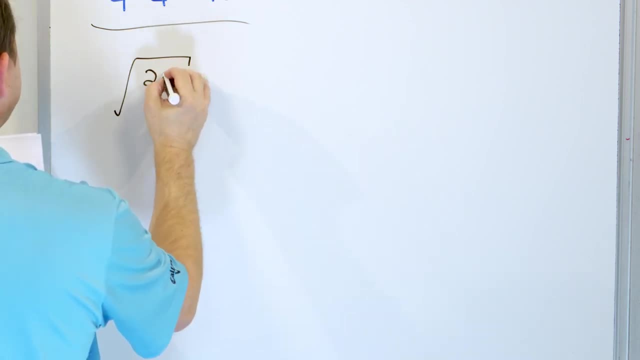 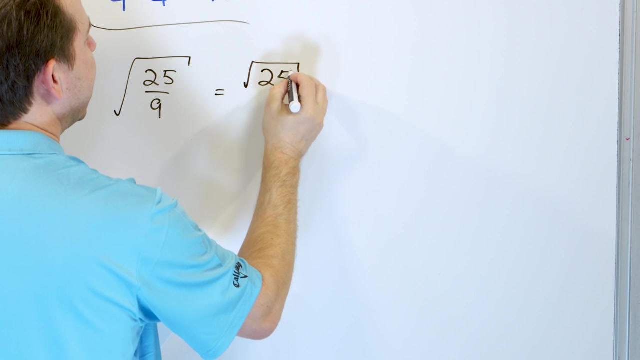 All right, let's take the square root: 25 over 9.. Again, you could write it as a fractional exponent if you want, but instead we'll just cut to the chase and say: well, that radical gets applied to the numerator and to the denominator. 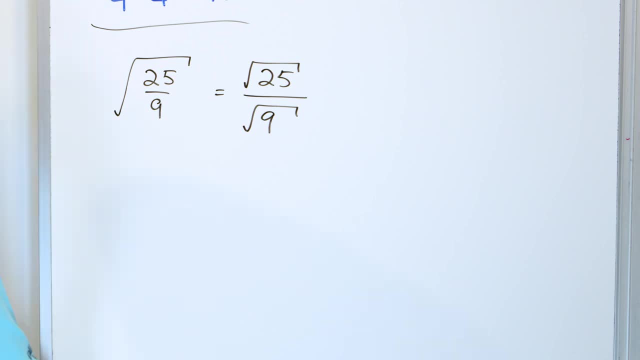 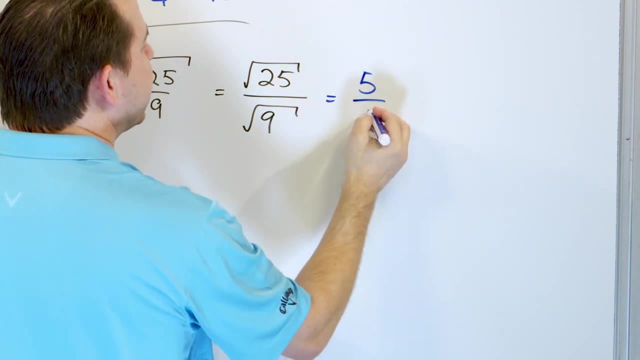 because they're really exponents. That's why they're allowed to do that. Now, the square root of 25 is 5, because 5 times 5 is 25, and the square root of 9 is 3, because 3 times 3 is 9.. 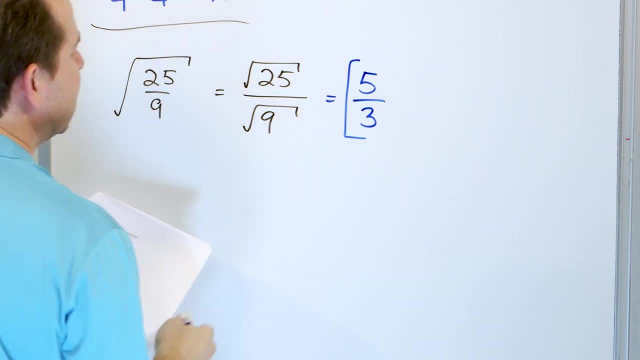 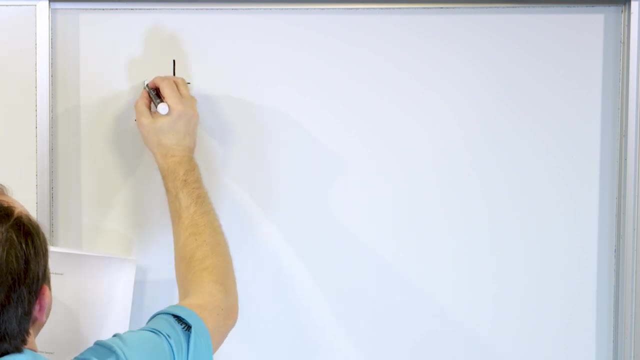 So 5-thirds. So you could write this as a mixed number if you want, but I'm just going to leave it like this. Let's take a look at something a little different. 1-27th, But not the square root, the cube root. 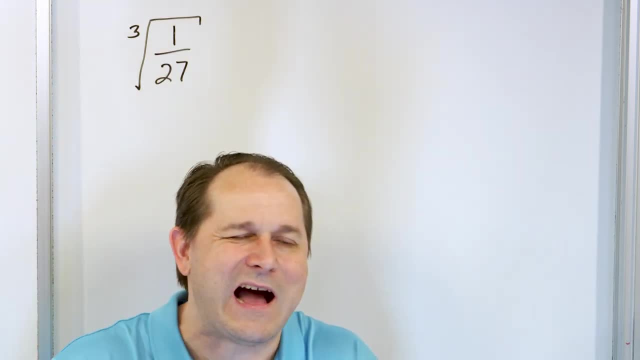 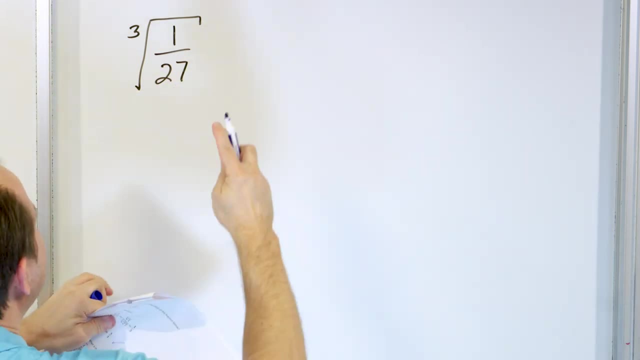 And even though the point of this lesson, the thrust of this lesson, is not the fractional exponents- I mean, that's not the point, but I don't think it's a hard concept. So I'm just telling you that this cube root thing can be written as an exponent: 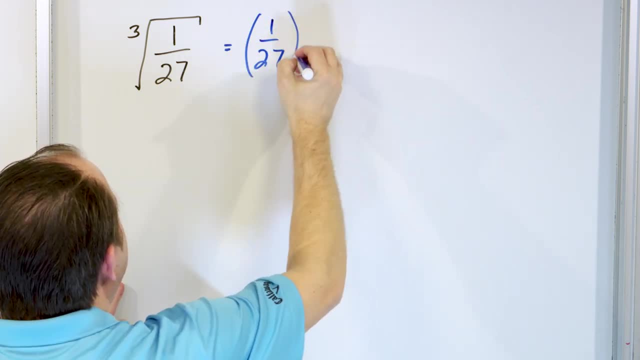 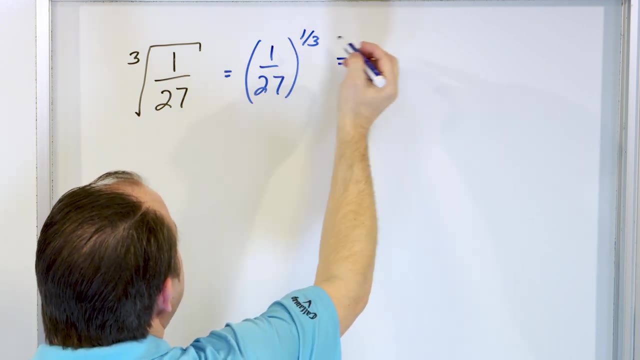 1 over 27.. If the square root is a half exponent, then the cube root is actually 1-third of an exponent. Exponents apply to the numerator and the denominator, So 1 to the 1-third and 27 to the 1-third. 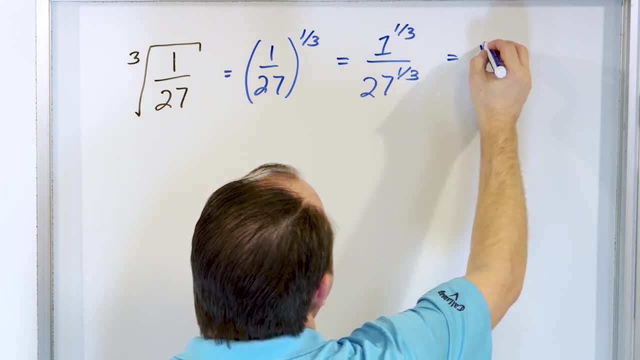 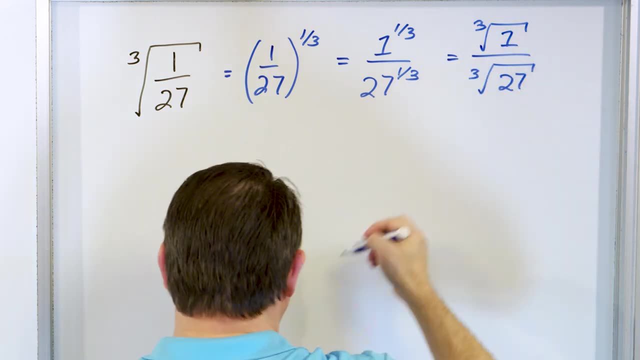 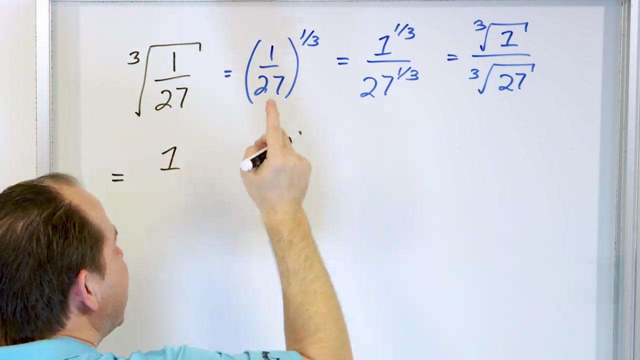 This exponent gets applied to the top and the bottom, but this 1-third power is the same thing as the cube root of 1. And it's the cube root of 27.. So what do we get? What's the cube root of 1? It is 1, because 1 times 1 times 1 is 1.. 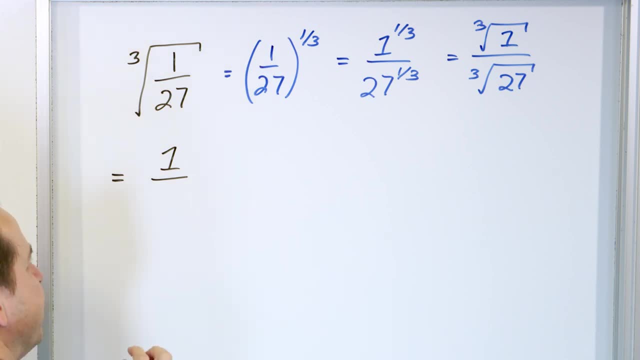 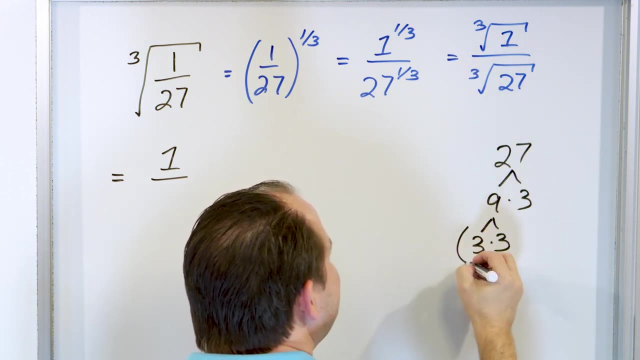 What's the cube root of 27?? You may not be totally sure. If you're not sure, do a factor tree: 27, 9 times 3, and then this 9 is 3 times 3.. We're looking for a cube root, so it has to be a triplet. 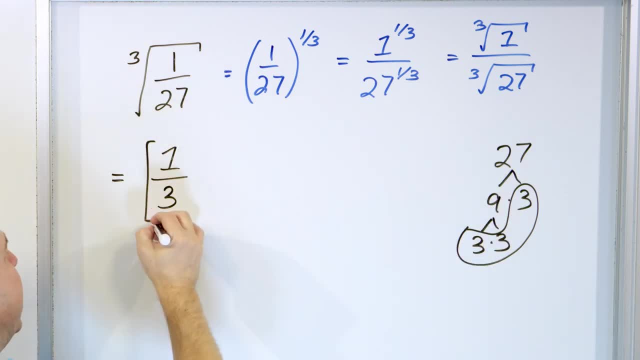 And that's all that's down there. so it comes out as a 3.. 3 is on the denominator, so the answer is 1-third. How do you know? Because that is correct. If you take 1-third times, 1-third times 1-third, all the 1s will multiply and give you 1.. 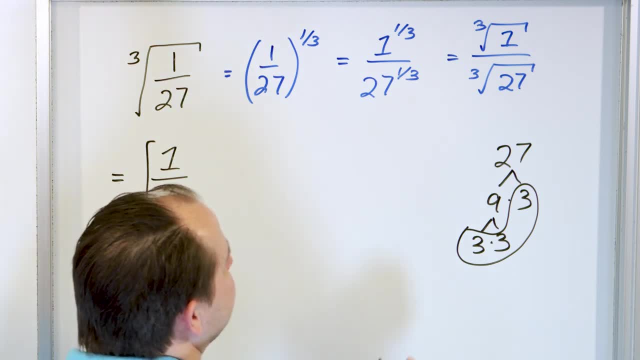 The 3 times 3 times 3 will multiply to give you 27, because 3 times 3 is 9.. And then 9 times the other 3 is 27, because even though I said I wouldn't check it, I guess I'll do it. 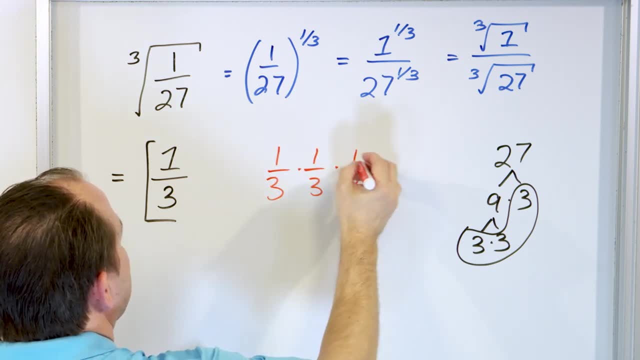 1-third, 1-third. 1-third, 1 times 1 times 1 is 1.. 3 times 3 is 9.. 9 times 3, 27.. And so it matches what you started with. 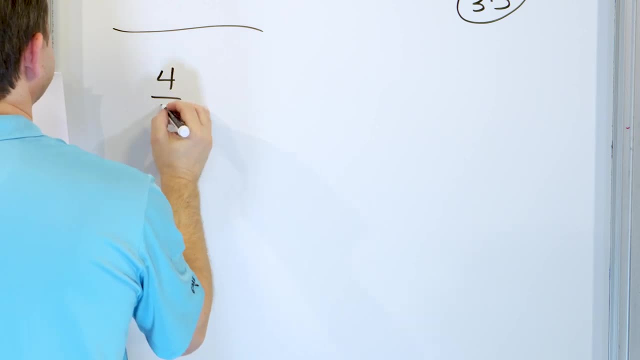 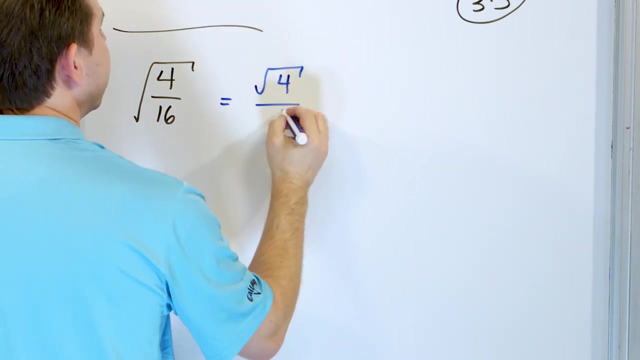 All right, only two more and we'll call it a day. What about 4-sixteenths? We're going to take the square root of that. So again, this radical can be applied to the numerator, can be applied to the denominator. 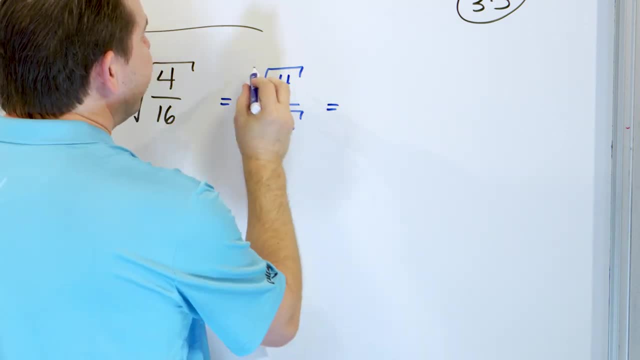 because it's basically an exponent, and it is an exponent. The square root of 4 is 2, because 2 times 2 is 4, and the square root of 16 is 4, because 4 times 4 is 16.. 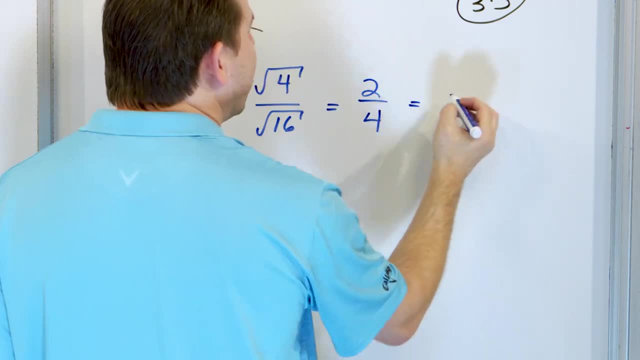 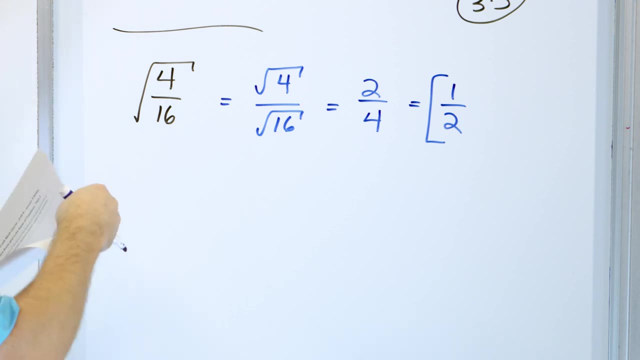 So you can leave it as 2-fourths or you can simplify it And 2-fourths reduces to 1-half. Just divide top and bottom by 2.. So 1-half is probably the simplest best answer to write down for this. 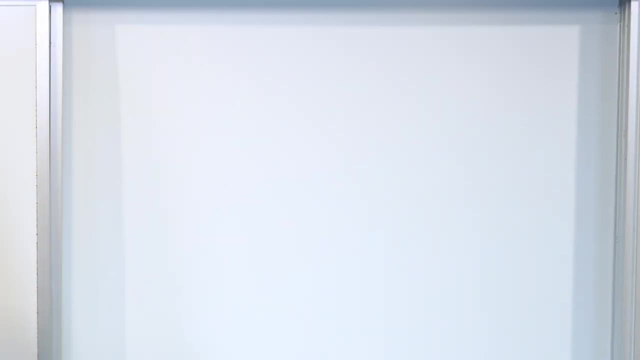 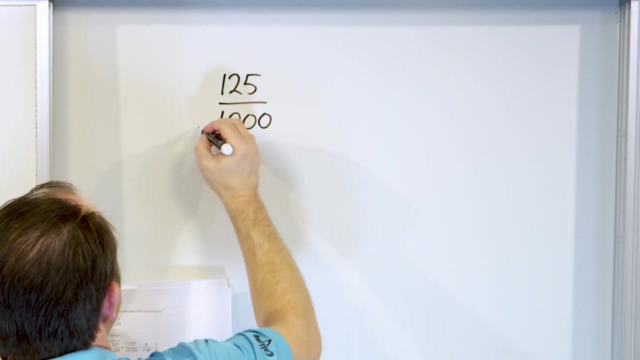 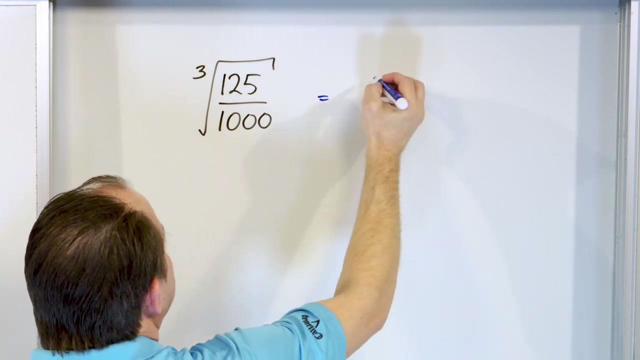 All right, we have one more And then we're done. Let's take a look at 125- over 1,000, and we're going to take the cube root of this, All right. so what we have is this: radical is a cube root. 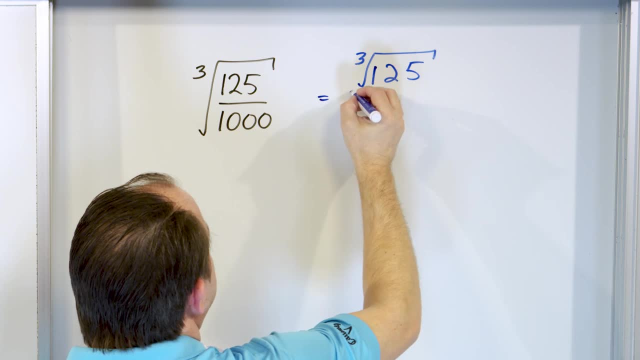 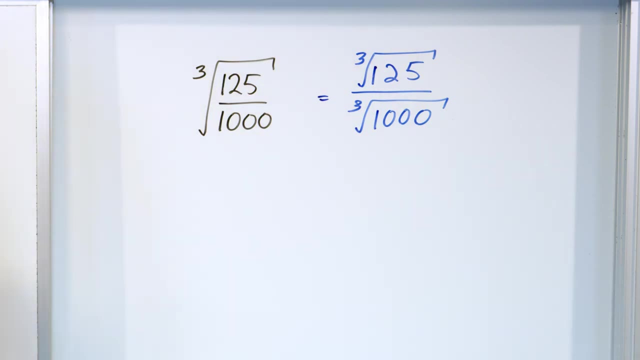 It's going to be applied to the numerator cube root of this guy And 1,000 is on the bottom and it's going to be applied to the denominator. So we have two different cube roots to figure out. Now it's better to go off to the side and just take 125 and figure out that is a cube root. 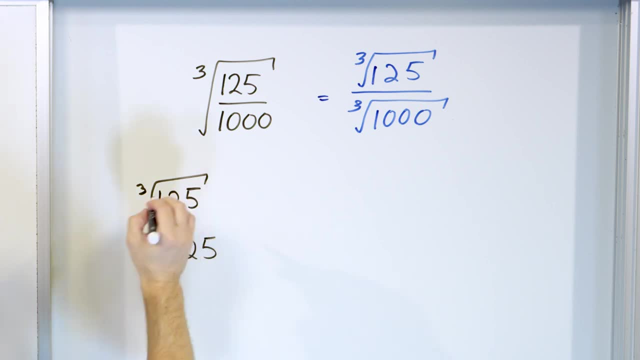 Well, we know that. 5 times 25.. That's 125.. And this 5 times 5,- if I can write 5 correctly, We're looking for triplets, so we have a triplet of 5.. That's all that we have. 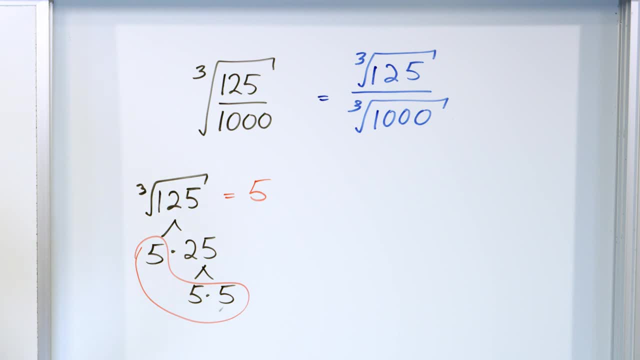 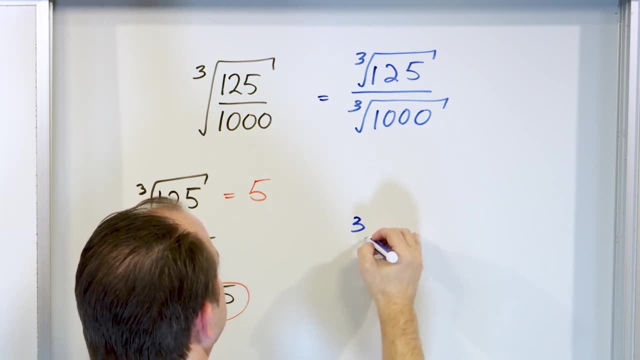 So the answer to this top radical is just 5.. And on the, I guess I'll go down below, On the bottom here, I guess I'll go, Yeah, I guess I'll go here. The cube root of 1,000, I'm going to write it as 10 times 100. 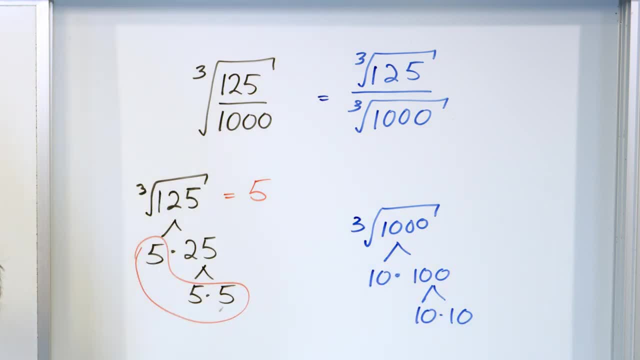 And I'm going to write this as 10 times 10.. I have a triplet Now on the bottom, the 10s, because it's a cube root. this is going to be 10.. So what we figured out is: the cube root of 125 is 5, and the cube root of 1,000 is 10.. 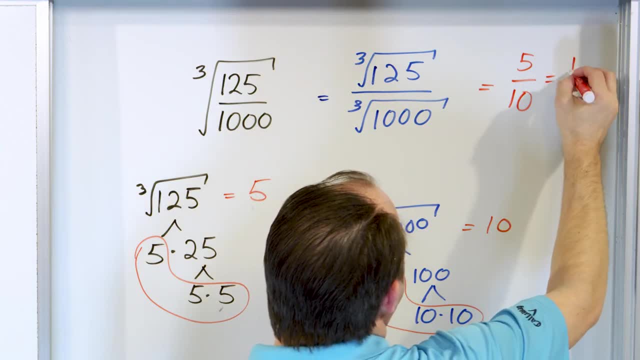 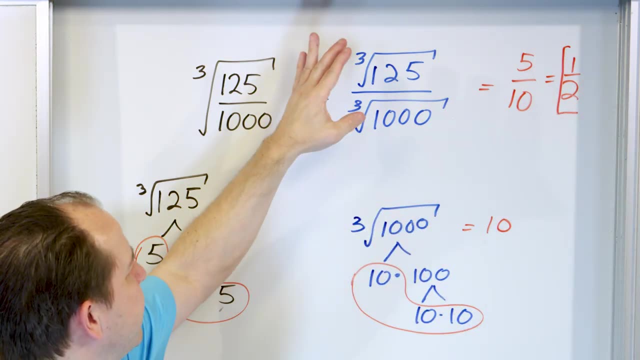 And you can divide top and bottom by 2 on this fraction and you're going to get again 1 half. So the answer to this simplest form is 1 half. When you have kind of cube roots, square roots that are kind of hard to do in your head. 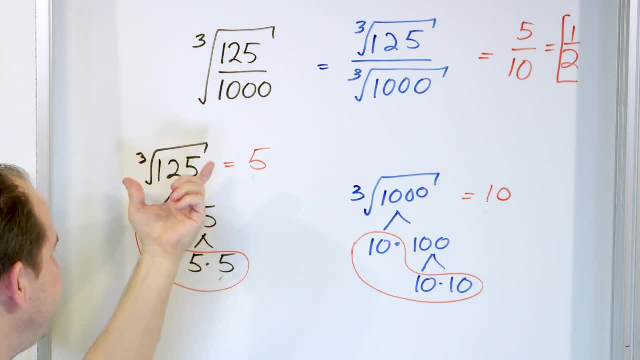 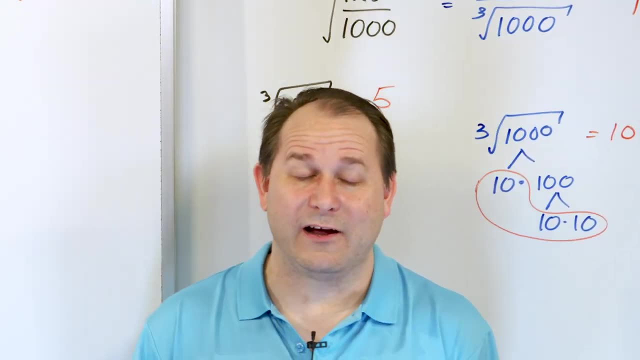 instead of trying to fit it all on one line, just go off to the side and figure this one out. Figure this one out, put it back into the answer so you don't make any mistakes. All right, So here we've talked about a lot actually. 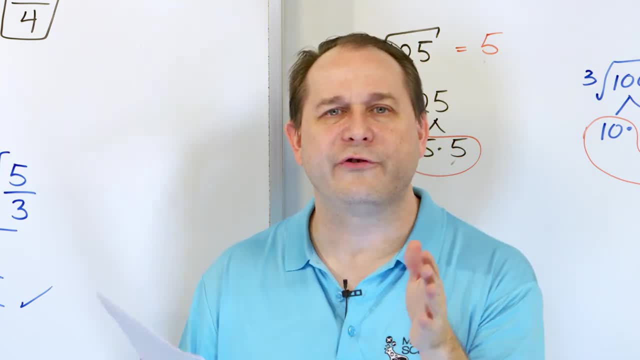 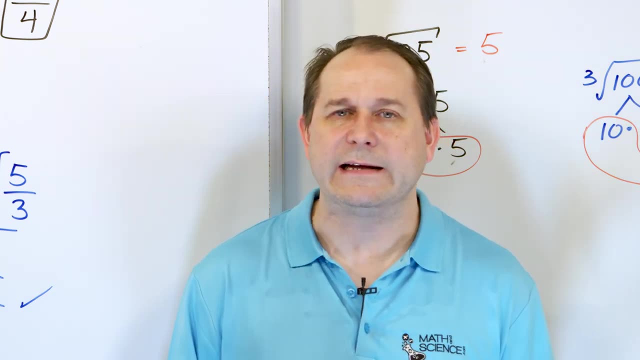 We've talked about how to apply square roots and cube roots to fractions And we said: hey, you can apply it to the numerator and then separately to the denominator and calculate the answer. I could have just left it like that and said: do it? 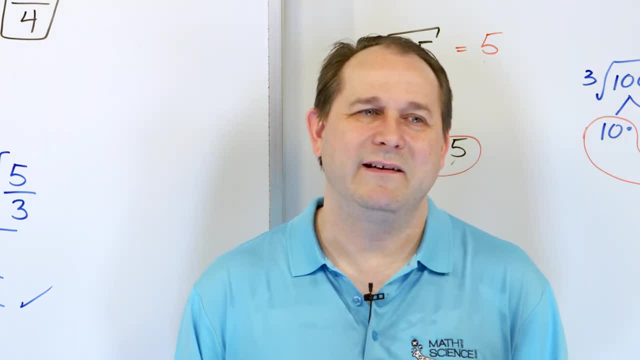 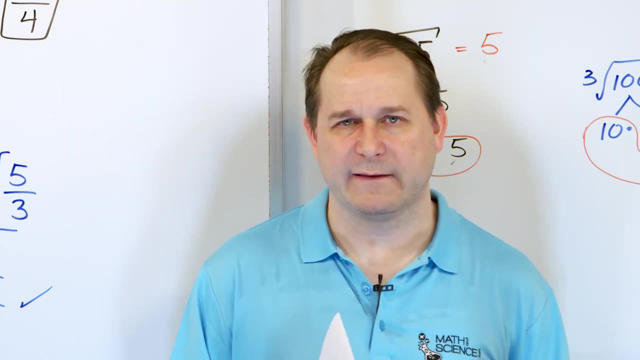 Trust me, I'm right and you've got to learn from me. But that's not great, because then you think all these rules are coming from nowhere. So I do a little aside and I say, hey, this isn't the thrust of the lesson.